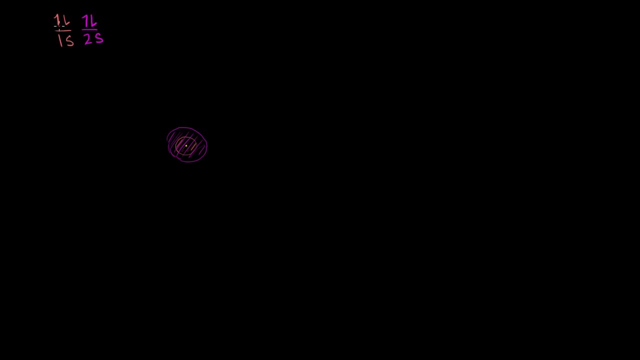 And I drew these arrows upward and downward, because the first electron that goes in the 1s orbital has one spin, and then the next electron to go into the 1s orbital will have the opposite spin, And so they keep pairing up in that way. 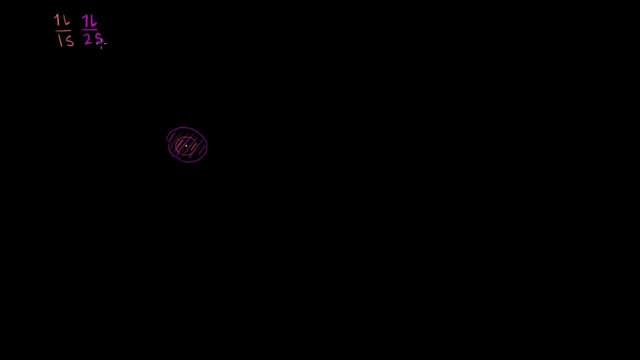 They have opposite spins. Now, if we keep adding electrons, now we move to the 2p orbitals, We move to the 2p And there's actually- you can view it as there are- three 2p orbitals. 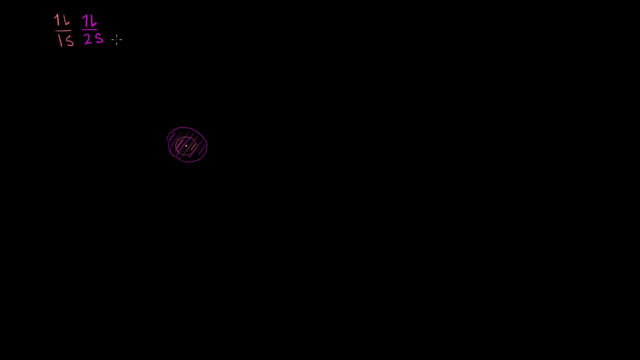 and each of them can hold two electrons. So we can hold a total of six electrons in the 2p orbitals, And let me draw them for you just so you can visualize it. So if we were to label our axes here, so think in three dimensions. 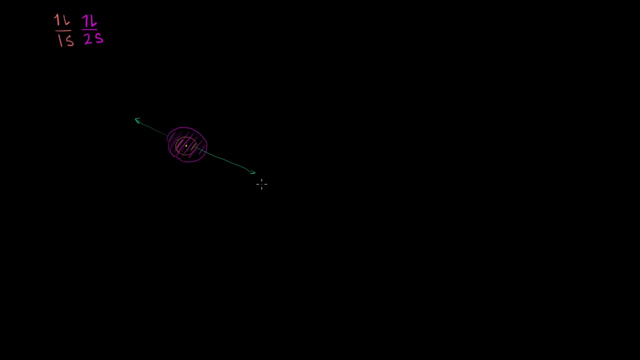 So imagine that that right there is the x-axis, That is our x-axis. Let me do this in different colors. Let's say that this right here is our y-axis, That is our y-axis, And then we have a z-axis. 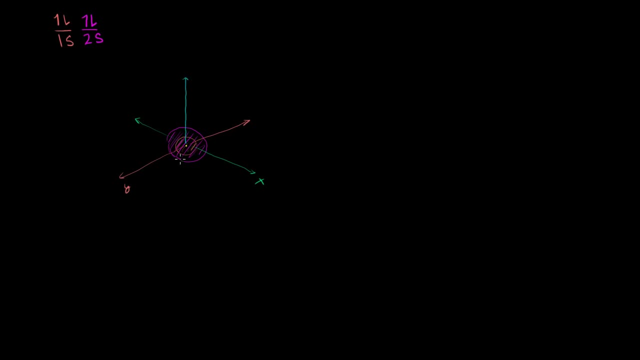 I'll do that in blue. So let's say we have a z-axis, just like that. You actually have a p orbital that goes along each of those axes, So you could have your. so let me do it. So you have your two. let me do this in a. let me do it in the same colors. 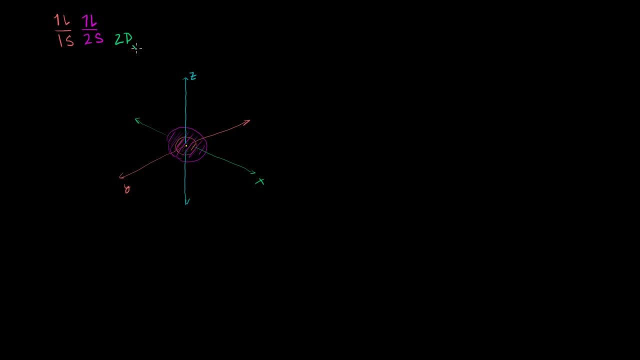 So you have your 2p sub x orbital, And so what that'll look like is a dumbbell shape that's going in the x direction. So let me draw my best attempt at drawing this. So it's a dumbbell shape that goes in the x direction, in kind of both directions. 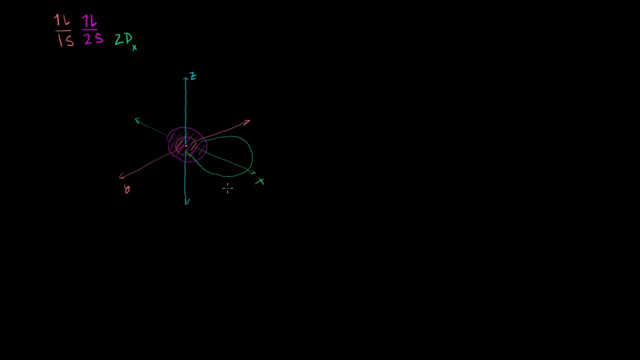 And it's actually symmetric. I'm drawing this end bigger than that end, So it looks like it's coming out at you a little bit, But let me draw it a little bit. better than that Can do a better job And maybe it comes out like that. 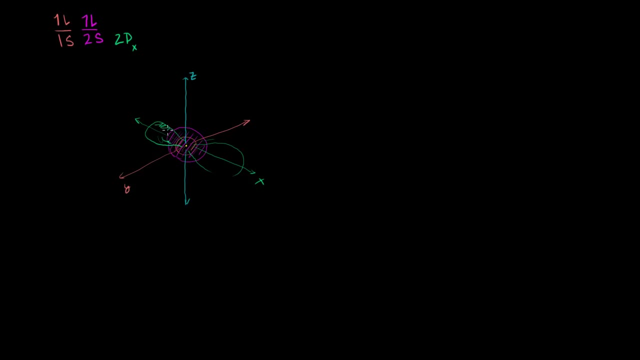 And remember, these are really just probability clouds But it's helpful to kind of visualize them as maybe a little bit more things that we would see in our world. But I think probability clouds is the best way to think about it. So that is the 2px orbital. 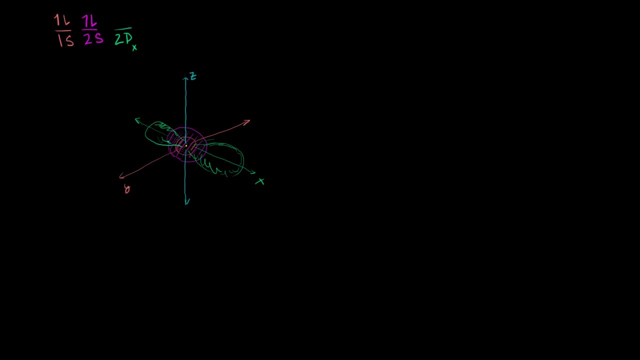 And then I haven't talked about how they get filled yet. But then you also have your 2py orbital Going in this axis, But same idea, Kind of a dumbbell shape in the y direction, Going in both along the y axis. 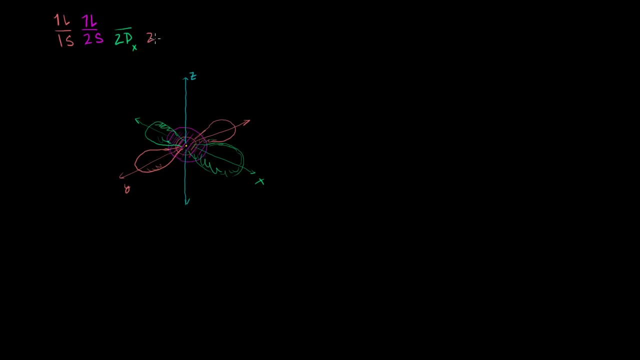 Going in that direction, and in that direction, Then of course, so let me do this 2py, And then you also have your 2pz, You also have your 2pz, And that goes in the z direction Up, like that. 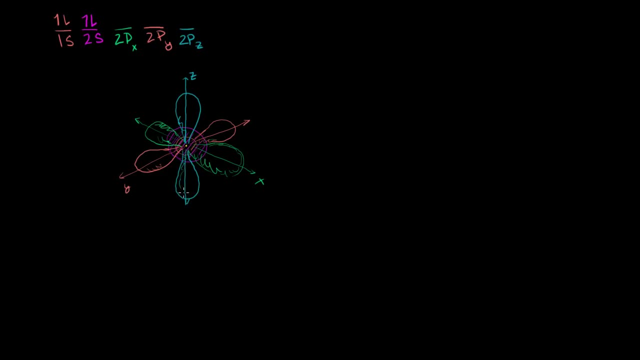 And then downwards like that. So when you keep adding electrons- So far we've added four electrons- If you add a fifth electron, If you add a fifth electron, You would expect it to go into the 2px, The 2px orbital, right there. 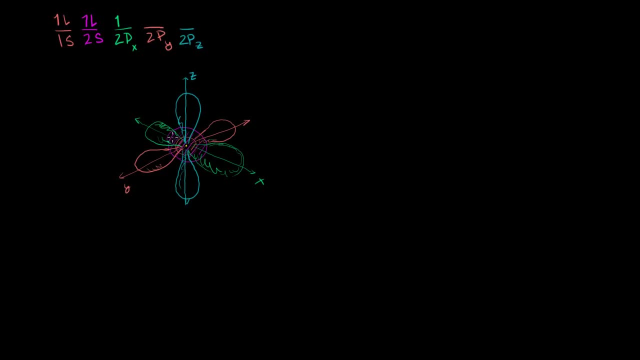 So even though this 2px orbital can fit two electrons, The first one goes there. The very next one won't go into that one. It actually wants to separate itself within the p orbital. So the very next electron that you add won't go into 2px. 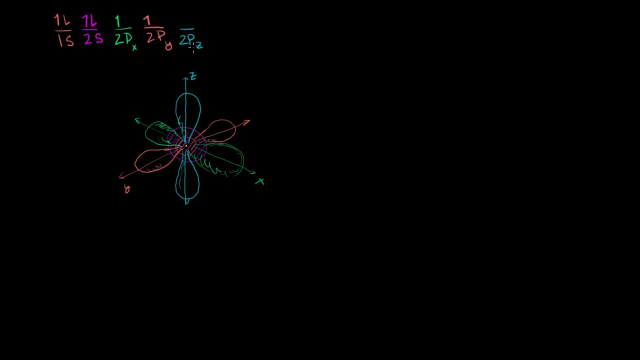 It'll go into 2py, And then the one after that won't go into 2py or 2px, It'll go into 2pz. They try to separate themselves And then if you add another electron, If you add, let's see. 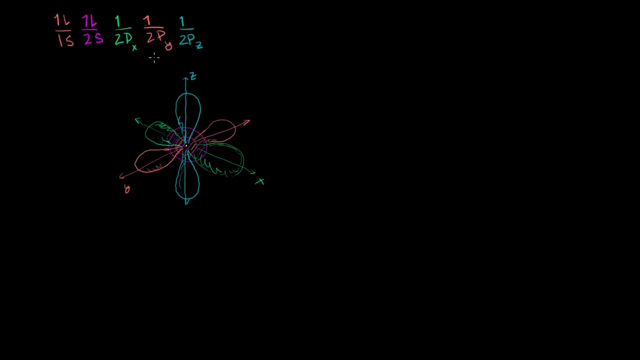 We've added one, two, three, four, five, six, seven. If you add an eighth electron, That will then go into the 2px orbital. So the eighth electron would go there, But it would have the opposite spin. 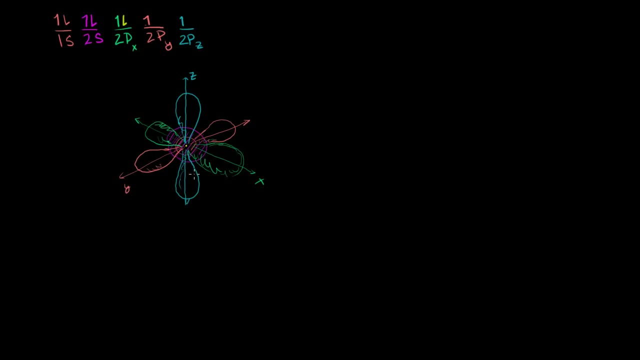 So this is just a little bit of review With a little bit of visualization. Now, given what we just reviewed, Let's think about what's happening with carbon. Carbon has six electrons. It's electron configuration It is 1s2.. 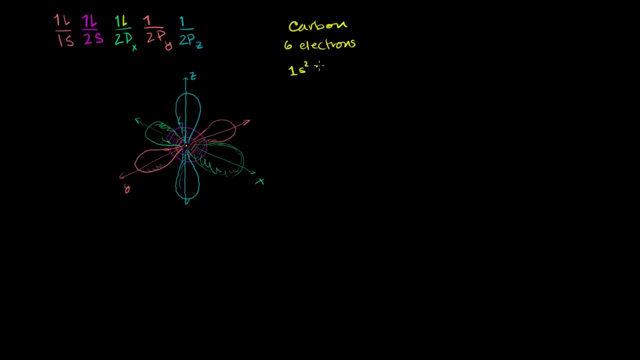 Two electrons in the 1s orbital, Then 2s2.. Then 2p2.. It only has two left because it has a total of six electrons. Two go here, Then there, Then two are left to fill the p orbital. 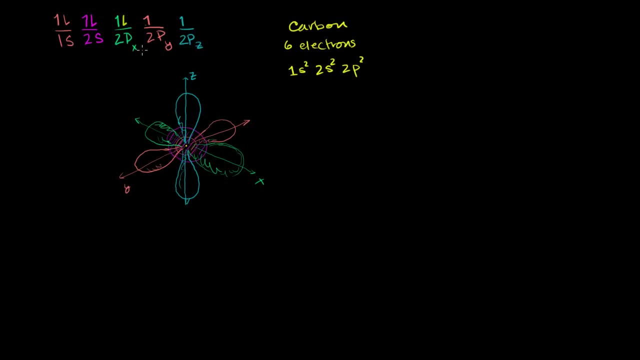 So if you go based on what we just drew And what we just talked about here, What you would expect for carbon, What you would expect for carbon, Let me just draw it out the way I did this. So you have your 1s orbital. 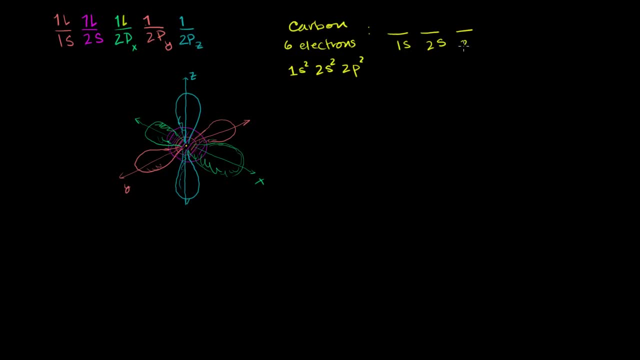 Your 2s orbital, And then you have your 2px orbital, Your 2py orbital And then you have your 2pz orbital. If you just go straight from the electron configuration, You would expect carbon. So the 1s orbital fills first. 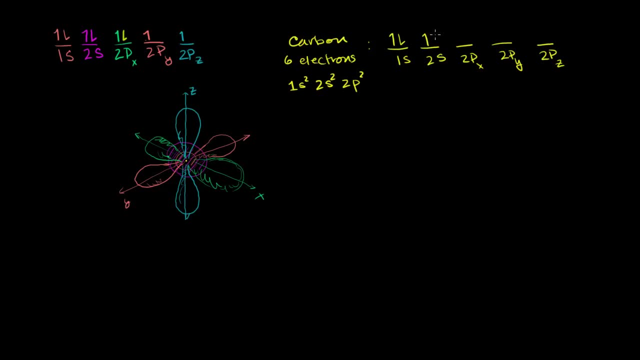 That's our first electron, Our second electron, Our third electron And then we go to our 2s orbital. That fills. next Third electron, Then fourth electron, Then you would expect maybe your fifth electron to go in the 2px. 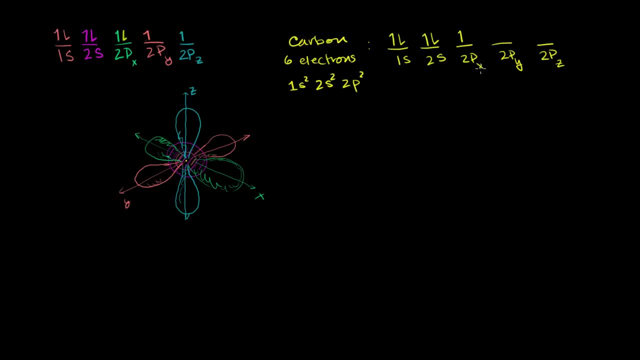 We could have said 2py or 2z, It just depends on how you label the axes. But you would have your fifth electron go into one of the p orbitals And then you would expect your sixth to go into another. So you would expect that to be kind of the configuration for carbon. 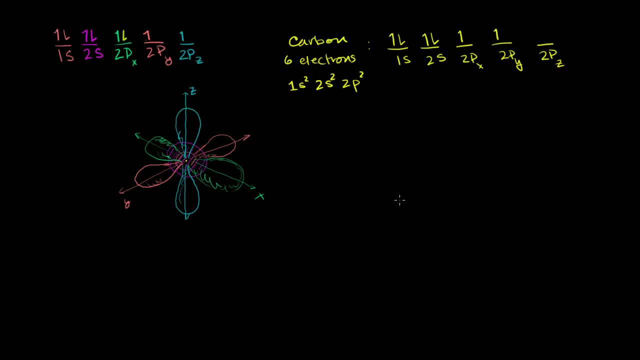 And if we were to draw it? If we were to draw it, Let's draw our axes. So that is our y-axis, And then this is our x-axis. Let me draw it a little bit better than that. So that is the x-axis. 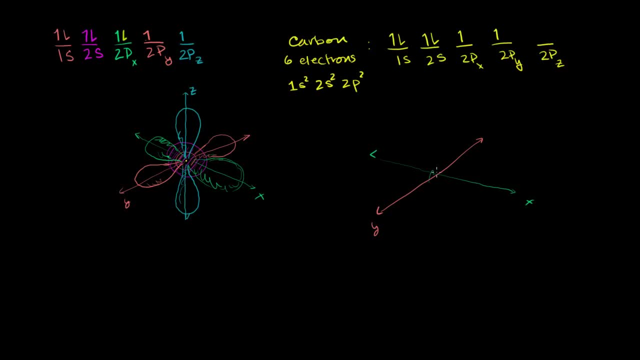 And of course you have your z-axis. You have to think in three dimensions a little bit, A little squiggly line there. Then you have your z-axis, Just like that. So first we fill the 1s orbital. So if our nucleus is sitting here, 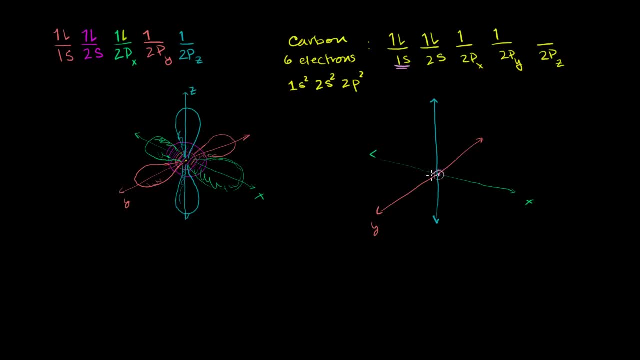 Our 1s orbital gets filled with two electrons. You can imagine that as a little cloud around the nucleus. Then we fill the 2s orbital And that would be a cloud around that, Kind of a shell around that, And then we would put one electron in the 2px orbital. 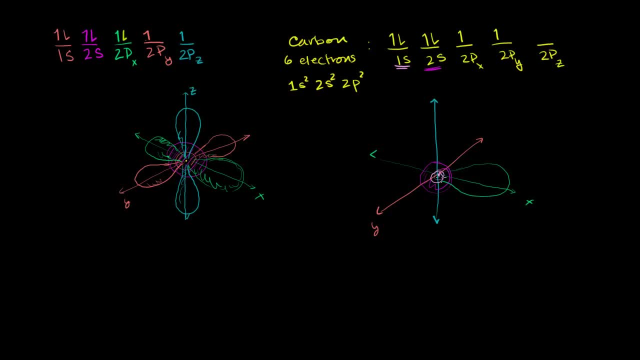 So one electron would start kind of jumping around or moving around, Depending on how you want to think about it, In that orbital over there 2px, And then you would have the next electron jumping around or moving around The 2py orbital. 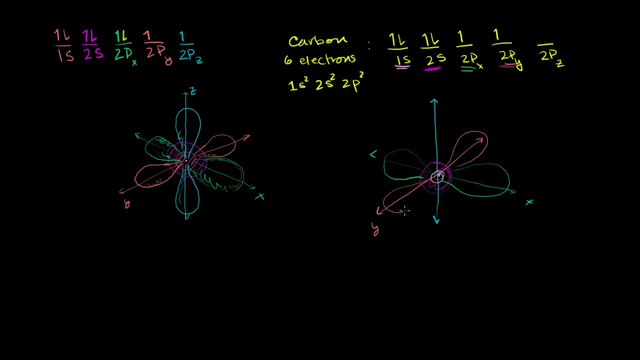 So it would be moving around like this And if you went just off of this, You would say: you know what These guys, This guy over here And that guy over there is lonely. He's looking for an opposite spin partner. 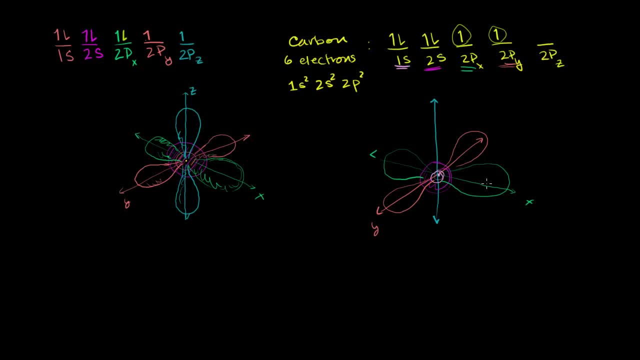 This would be the only places that bonds would form. You would expect some type of bonding to form with the x orbitals Or the y orbitals. Now, that's what you would expect if you, just straight up, kind of stayed with this model. 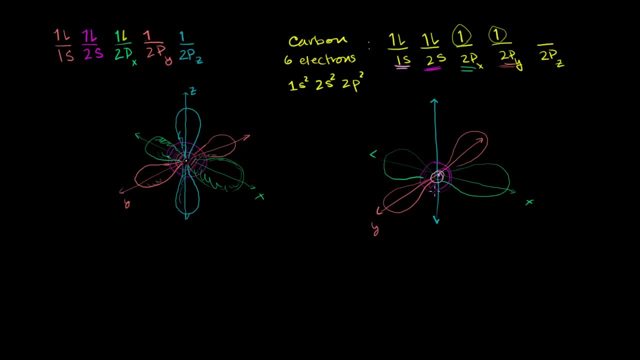 Of how things fill And how orbitals look. The reality of carbon- And I guess the simplest reality of carbon Is if you look at a methane molecule- Is very different than what you would expect here. With a methane First of all, what you would expect here. 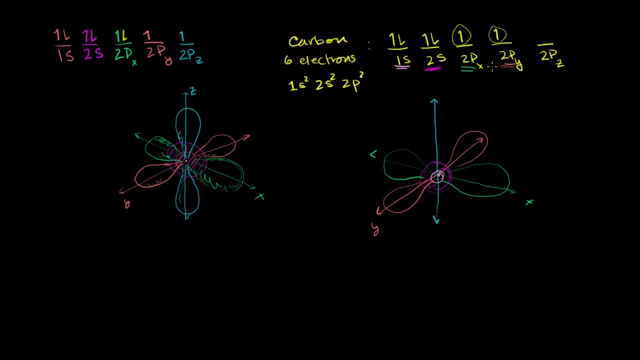 Is that carbon would probably, maybe It would form 2 bonds, But we know carbon forms 4 bonds. That it wants to fill it. It wants to pretend like it has 8 electrons. That, frankly, almost every atom wants to pretend like it has 8 electrons. 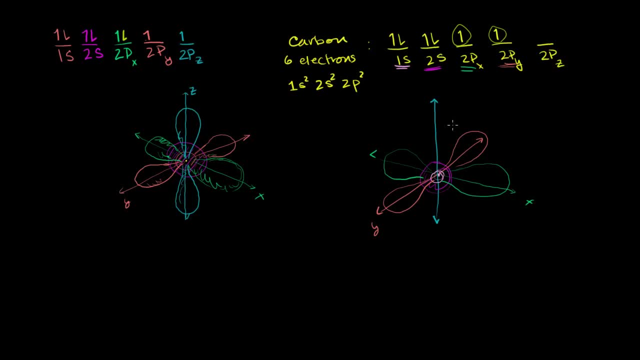 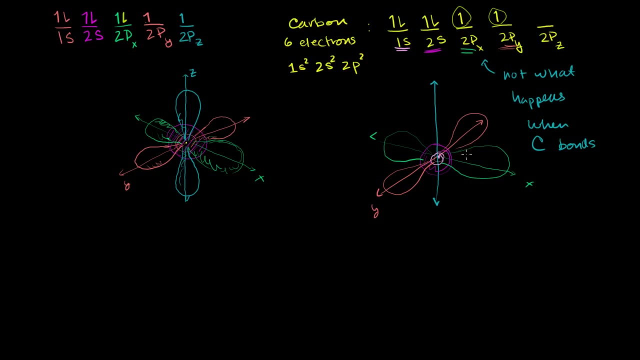 So in order for that to happen, You have to think about a different reality, And this isn't really what's happening when carbon bonds, So not what happens when carbon bonds, What's really happening when carbon bonds- And this will kind of go into the discussion of sp3 hybridization. 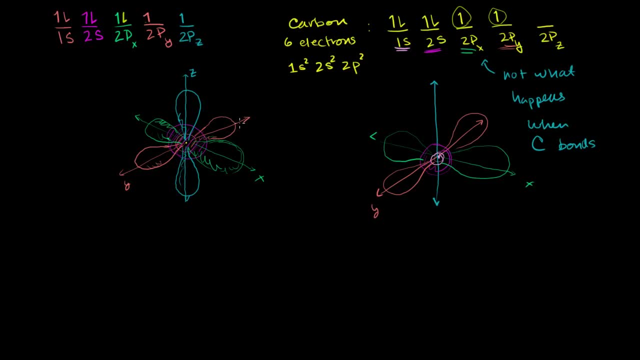 But what you're going to see is it's not that complicated of a topic. It sounds very daunting But it's actually pretty straight forward. What really happens when carbon bonds Wants to form 4 bonds with things Is it's configuration. 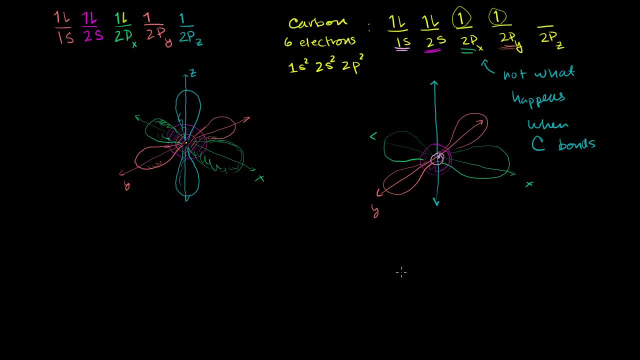 You can imagine, looks more like this. It looks more like this: So you have 1s And we have 2 electrons there, And then you have your 2s, 2px, 2py And 2pz. 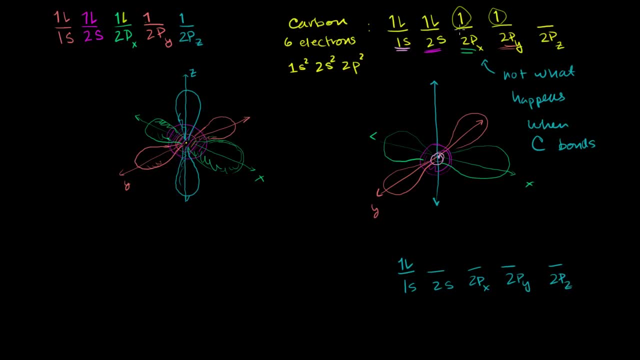 Now what you can imagine is it wants to form 4 bonds. It has 4 electrons that are willing to pair up with electrons from other molecules. In the case of methane, That other molecule is a hydrogen. So what you can imagine is: 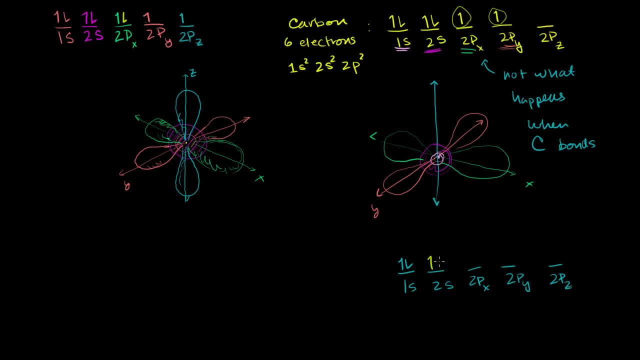 Is that the electrons actually Maybe the hydrogen attracts? this Brings this electron right here into a higher energy state And puts it into 2z. That's one way to visualize it. So this other guy here maybe ends up over there. 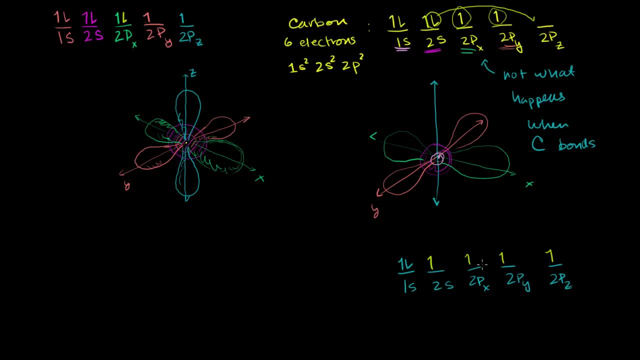 And then these 2 guys are over there and over there. Now, all of a sudden, it looks like you have 4 lonely guys And they are ready to bond, And that's actually more accurate of how carbon bonds It likes to bond with 4 other people. 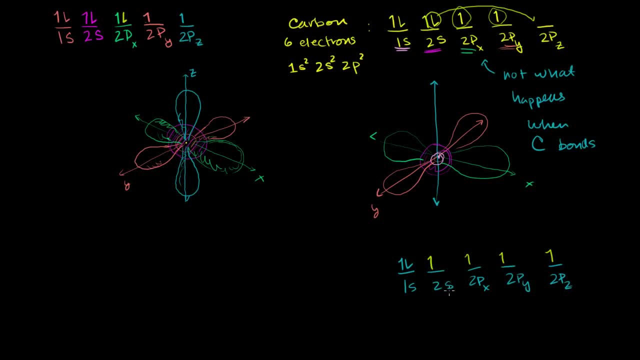 Now It's a little bit arbitrary Which electron ends up in each of these things. And even if you had this type of bonding, You would expect You would expect things to bond along the xy and z axis. The reality is The reality of carbon. 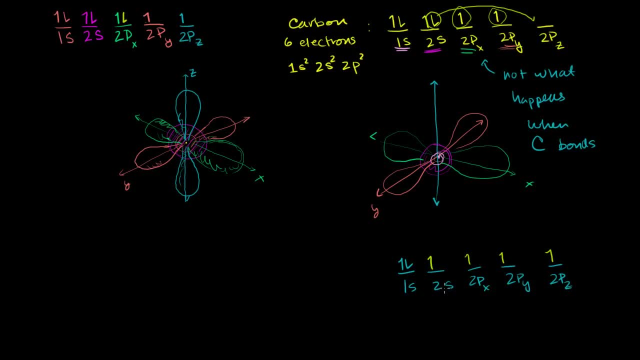 Is that these 4 electrons in its second shell Don't look like they're in. just You know, the first one doesn't look like it's just in the s orbital, And then the p's and y and z For the other 3.. 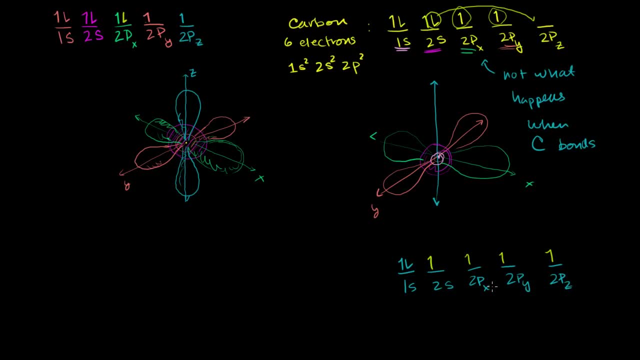 They all look like they're a little bit in the s And a little bit in the p orbitals, So let me, Let me make that clear. So, instead of this being a 2s, What it really looks like for carbon. 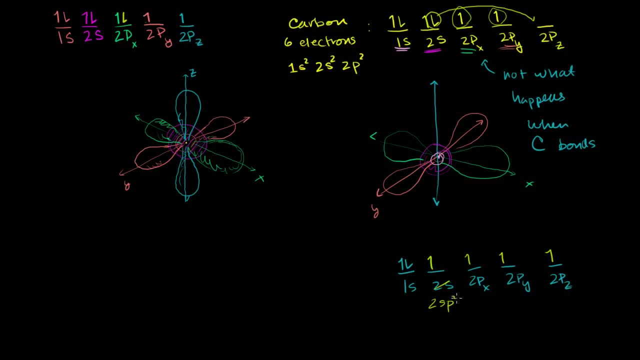 Is that. this looks like a 2sp3 orbital. This looks like a 2sp3 orbital. That looks like a 2sp3 orbital. That looks like a 2sp3 orbital. They all look like they're kind of in the same orbital. 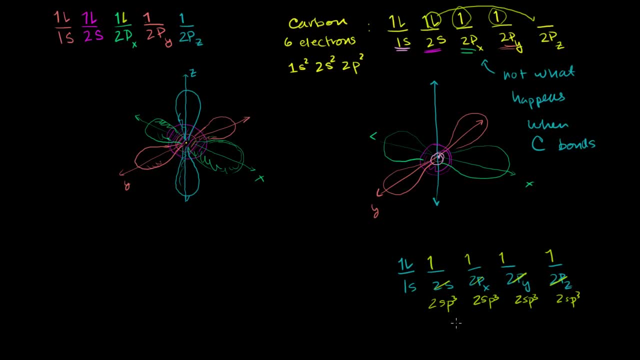 And this special type of You know it sounds very fancy, This sp3 hybridized orbital. What it actually looks like Is something that's in between an s and a p orbital. It has a 25% s nature And a 75% p nature. 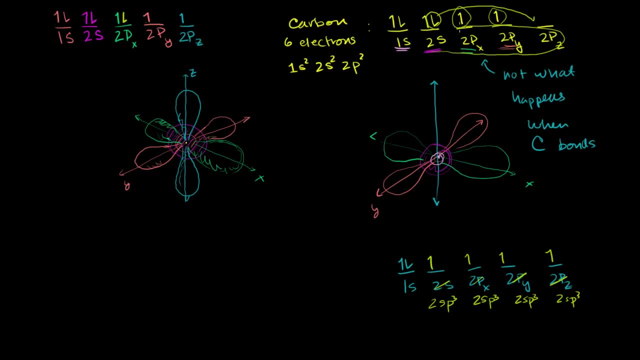 You can imagine it as being a mixture Of these 4 things. That's what. That's the behavior that carbon has. So when you mix them all, When you mix them all Instead of having a An s orbital. So if this is a nucleus, 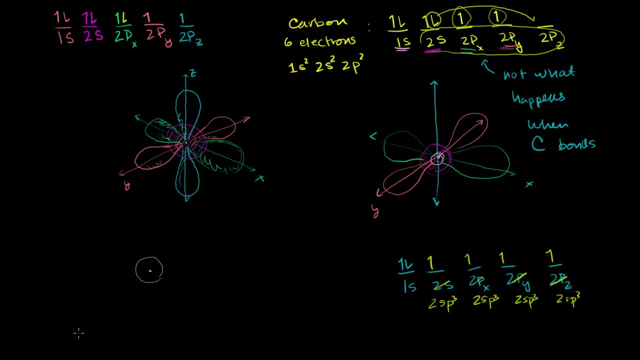 We do a cross section. An s orbital looks like That And a p orbital And a p orbital Looks something like that In cross section. When you So: this is a, Let me, This is an s And that is a p. 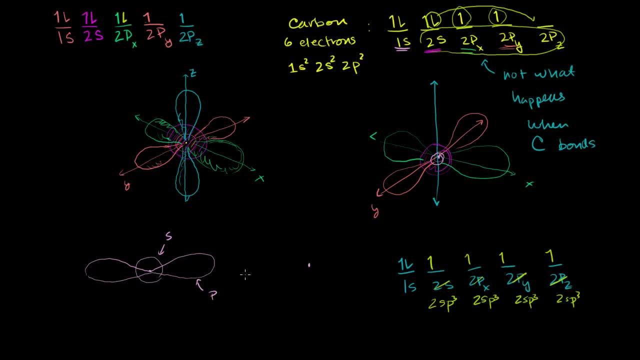 When they get mixed up, The orbital looks like this. An sp3 orbital Looks something like this. Looks something like this. This is an sp, A hybridized Sp3 orbital. Hybrid just means A combination of 2 things. 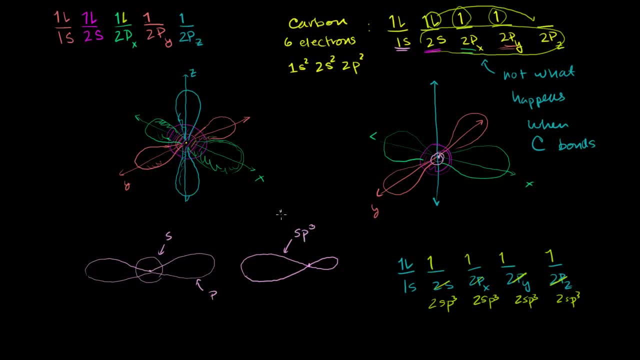 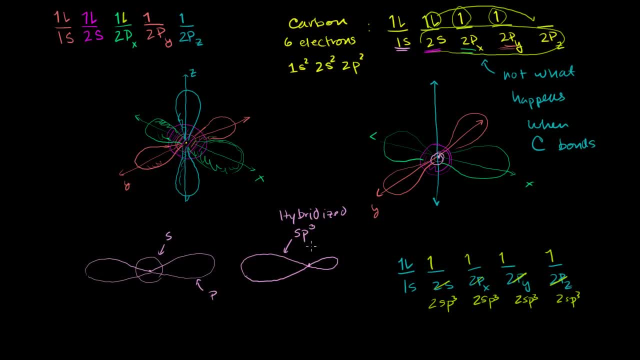 And p, And p And a hybridized sp3 orbitals are the orbitals when carbon bonds with things like hydrogen, Or really when it bonds with anything, And so if you look at a molecule of methane And you know people talk about high sp3 hybridized orbitals. 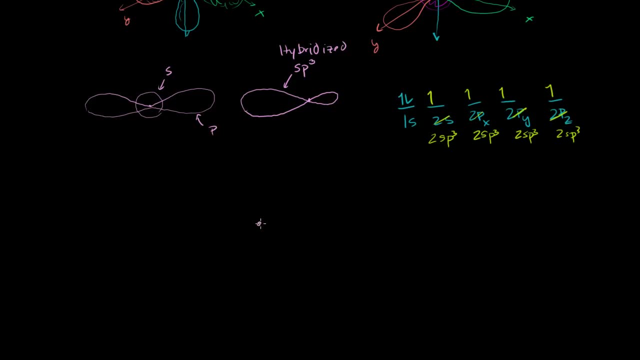 All they're saying is that you have a carbon in the center. Maybe I Let me draw the. Oh yeah, Let's say that's the carbon nucleus right there. And instead of having 1 s and 3 p orbitals, It has 4 sp3 orbitals. 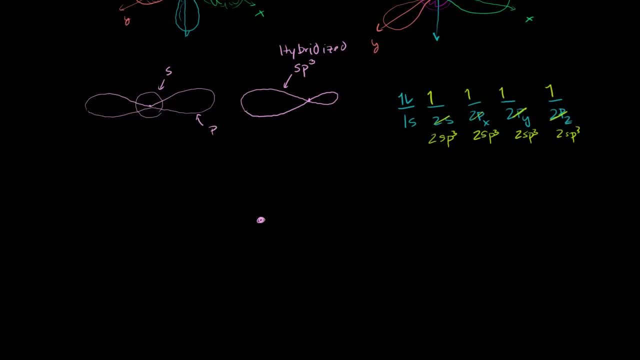 So let me try my best at drawing the 4 sp3 orbitals. So let's say that this is the big lobe That's kind of pointing near us And it has a small lobe in the back, And then you have another one that has a big lobe like that. 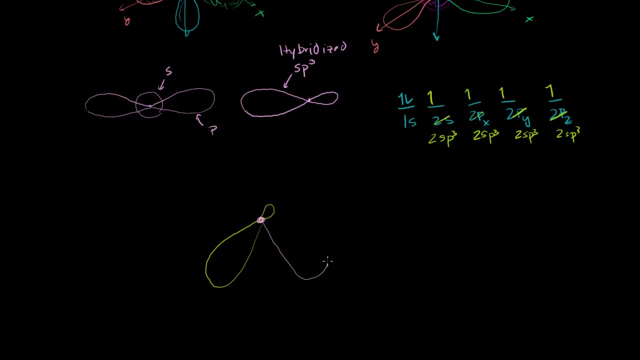 And a small lobe in the back, And then you have one that's going back behind the page. So let me draw that So you can kind of imagine a 3 legged stool, And then it's small lobe will come out like that. 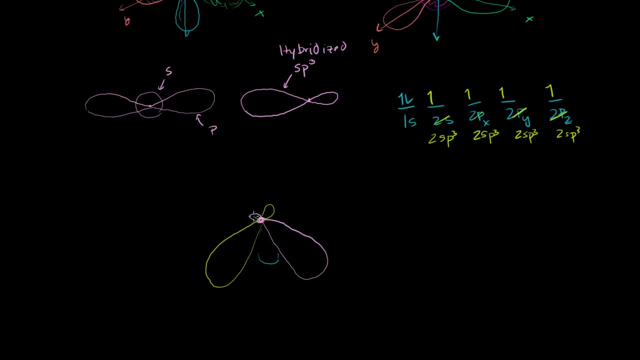 And then it's going to the back, And then it's going to the back, And then it's going to the back, And then it's going to come out like that, And then you have one where the big lobe is pointing straight up. 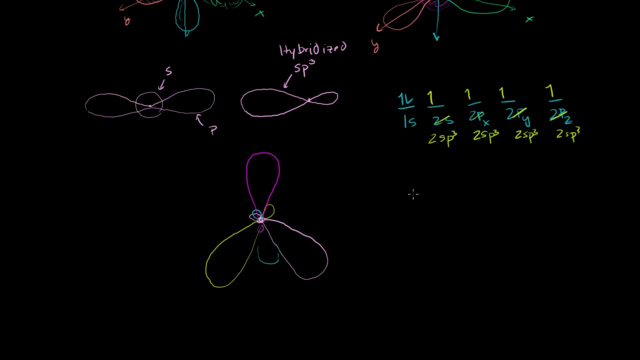 The big lobe is pointing straight up And it has a small lobe going down. You can imagine it's kind of a 3 legged stool. One of them is behind like that And it's pointing straight up. So 3 legged stool with something. 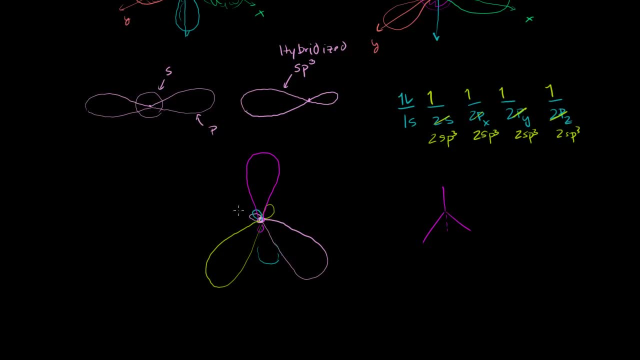 It's kind of like a tripod, I guess is the best way to think about it, And so that's the carbon nucleus in the center, And then you have the hydrogens, So that's our carbon right there, And then you have your hydrogens. 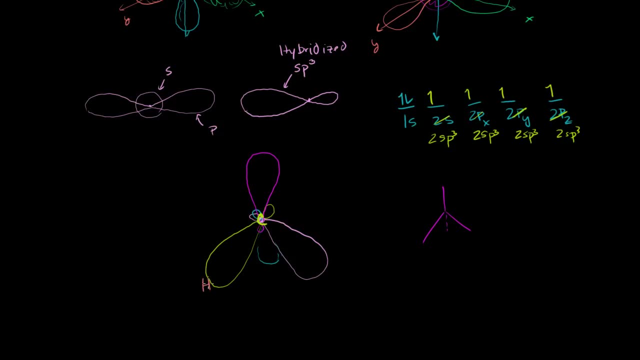 You have a hydrogen here. A hydrogen just has one electron in the 1s orbital. So the hydrogen just has 1s orbital. You have a hydrogen here, just has a 1s orbital. It has a hydrogen here, 1s orbital. 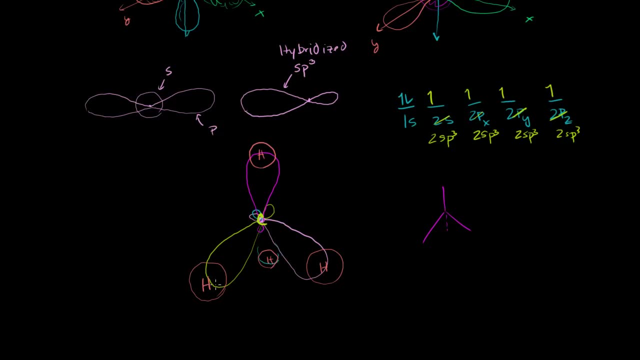 Hydrogen here 1s orbital. And so this is how the hydrogen orbital and the carbon orbitals get mixed: The hydrogen's 1s orbital bonds with, well, each of the hydrogen's 1s orbital bonds with each of the carbon's sb3 orbitals. 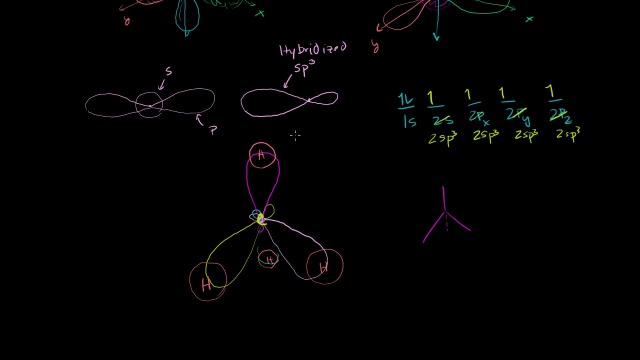 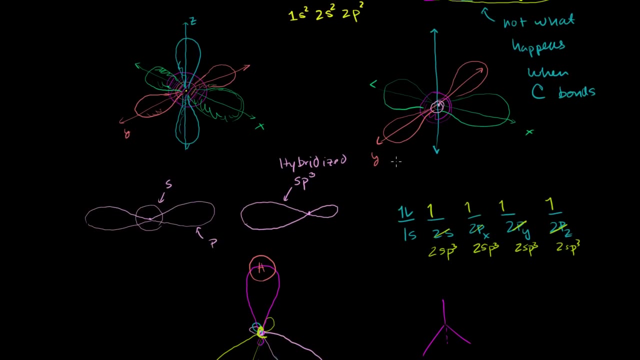 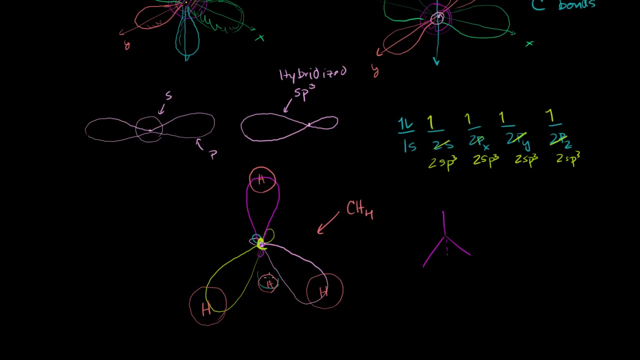 And just so you get a little bit more notation. so when people talk about hybridized sp3 orbitals, all they're saying is: look, carbon doesn't bond. when, once carbon, this right here is a molecule of methane. right, This is CH4, or methane. 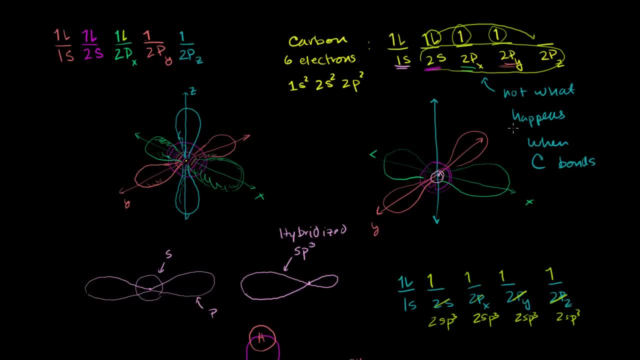 And it doesn't bond like you would expect. if you just went with straight vanilla s and p orbitals. If you just went straight vanilla sp orbitals, the bonds would form. maybe the hydrogen might be there and there, and if it had four hydrogens, maybe there and there. 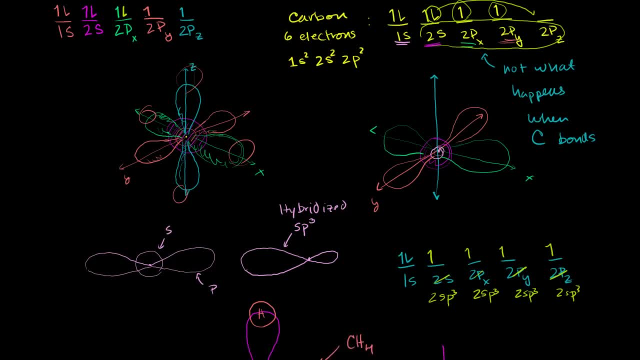 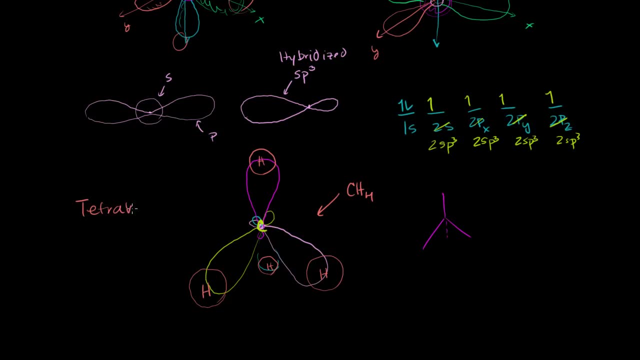 depending on how you want to think about it, But the reality is it doesn't look like that. It looks more like a tripod. It has a tetrahedral shape, And the best way that that can be explained, I guess, the shape of the structure is: if you have four, equally four of 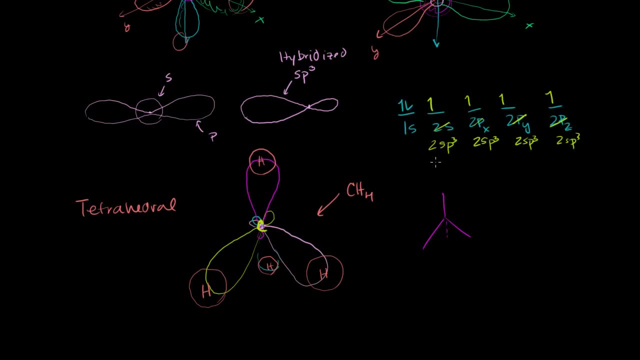 the same types of orbital shapes. And those four types of orbital shapes are hybrids between s's and p's. And one other piece of notation to know. sometimes people think it's a very fancy term, but when you have a bond between two molecules, where the orbitals are kind of 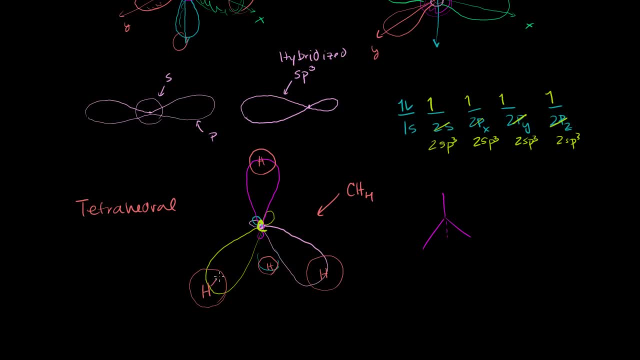 pointing at each other. So you can imagine: right here this hydrogen orbital is pointing in that direction, This sp3 orbital is pointing in that direction. They're overlapping right around here. This is called a sigma bond. Sigma bond We're kind of. the overlap is along the same axis, as if you. 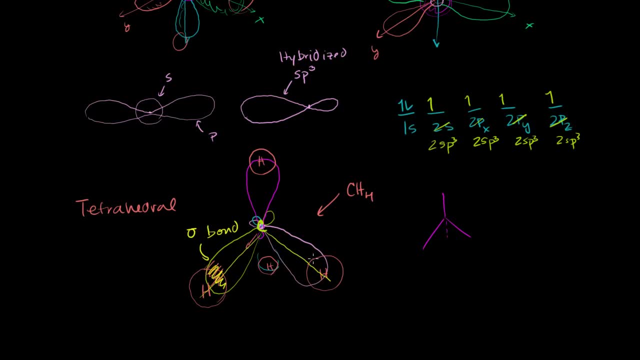 connected the two molecules. Over here you connect the two molecules. the overlap is on that same axis. This is the strongest form of covalent bonds And this will be a good basis for discussion, maybe in the next video when we talk a little bit about pi bonds. 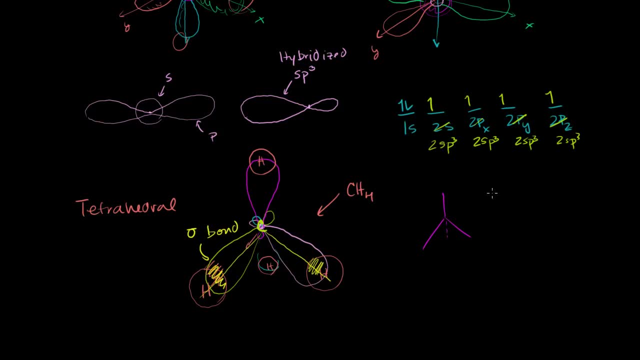 But the big takeaway of this video is just to understand. what does it mean? what is a sp3 hybridized orbital? Nothing fancy, just a combination of s and p orbitals. It has 25% s-caracterization. It has 25% s-caracterization. 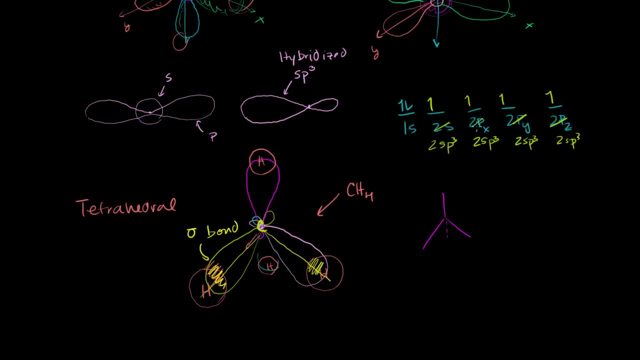 It has 25% p-character, 75% p-character, which makes sense, And it's what exists when carbon forms bonds, especially in the case of methane. That's what describes its tetrahedral structure. That's why we have an angle between the various branches of 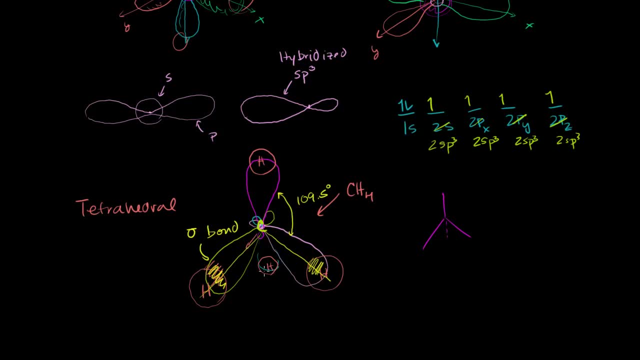 109.5 degrees, which some teachers might want you to know. so it's useful to know If you take this angle right here- 109.5, that's the same thing as that angle- Or if you were to go behind it, that angle right there, 109.5.